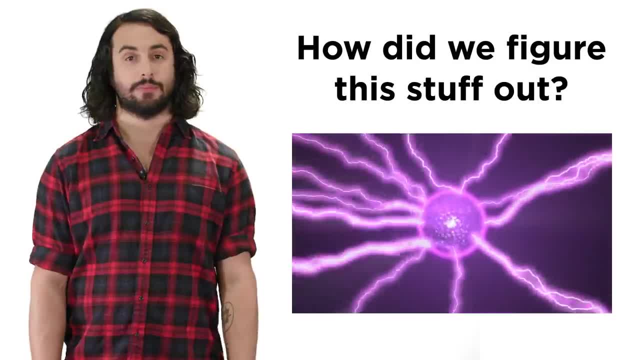 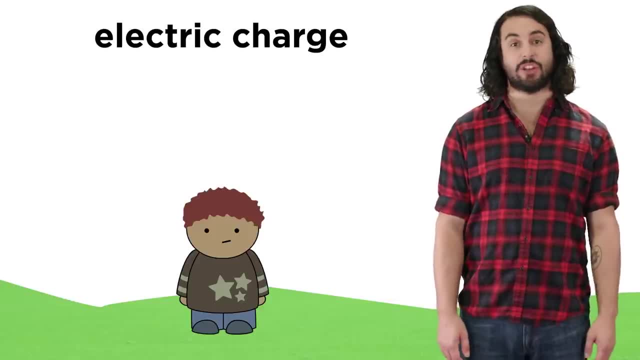 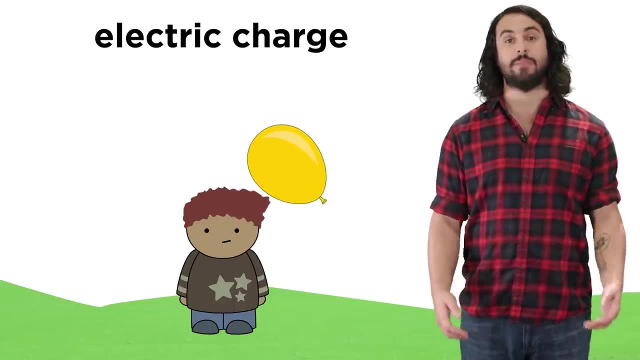 of this incredible power. So let's learn about it now. First, we noticed that there was such a thing as electric charge. The easiest demonstration of this involves rubbing a balloon on your hair and seeing how the balloon will then attract your hair by some mysterious force. 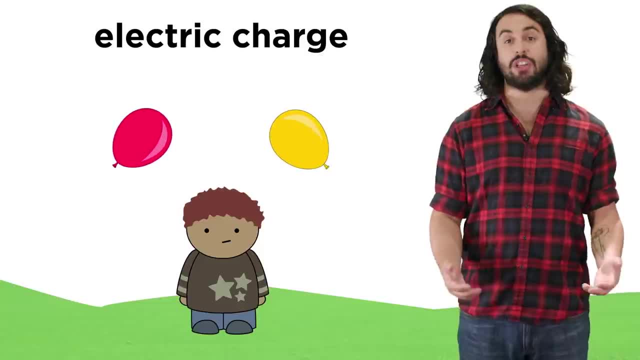 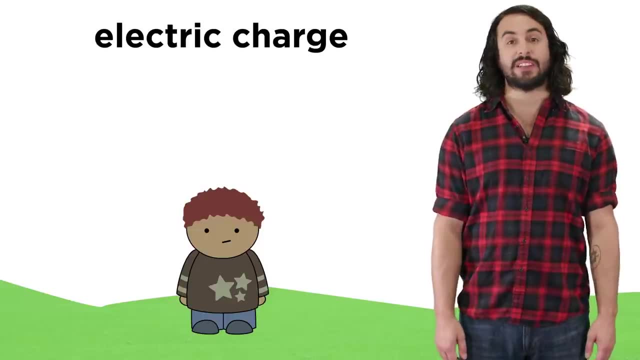 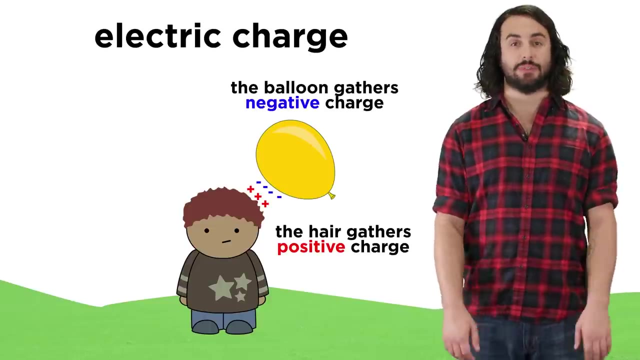 Two balloons that have been rubbed on your hair will strangely push each other away. This occurs because of electric charge, which is displaced by the rubbing together of these materials. The hair becomes positively charged and the balloons become negatively charged, which is terminology developed by Benjamin Franklin. 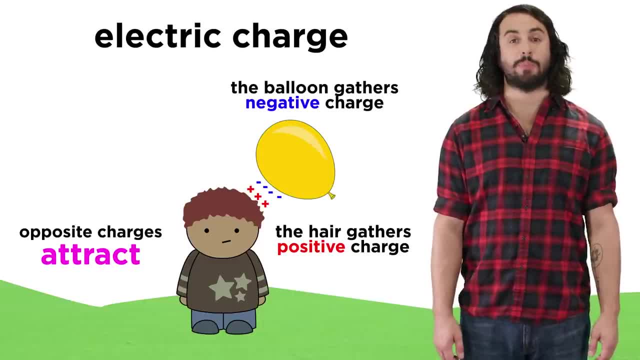 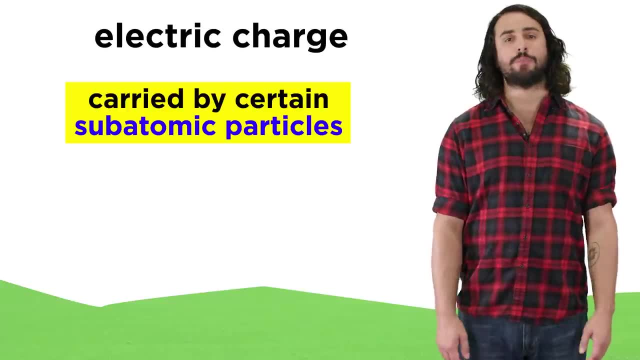 Opposite charges will attract one another, which is why your hair sticks to the balloon, and, like charges, repel, which is why the two balloons push each other away. This property of electric charge is carried by certain subatomic particles, the most common 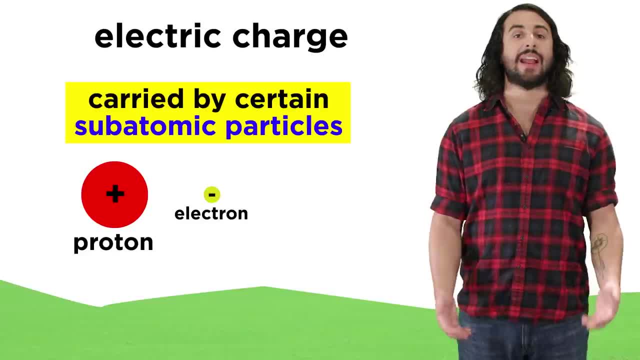 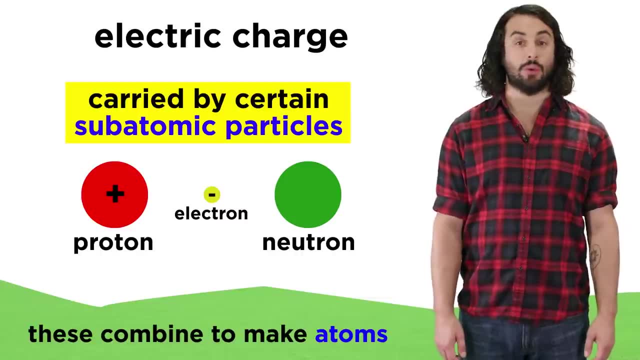 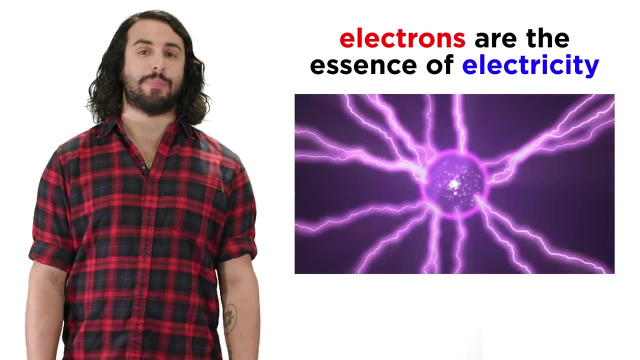 of these are protons, which are positive- These are positively charged- and electrons, which are negatively charged. Along with neutrons, these make up all the atoms in the universe. For more about atoms, check out my general chemistry course. As it happens, electrons, which are the essence of electricity, are easily transferable, and 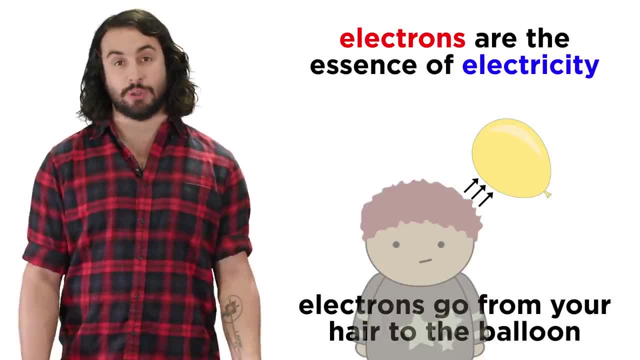 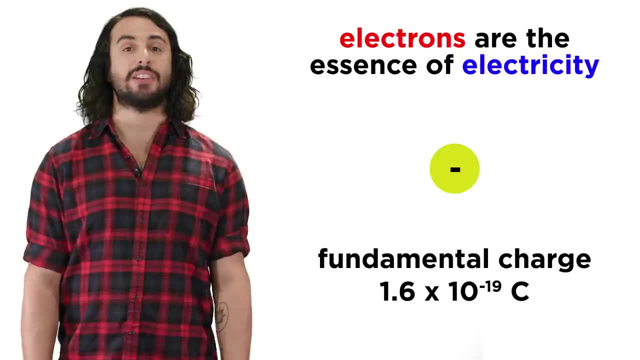 it is the transfer of electrons, in this case from your hair to the balloon, that generates electric charge. in previously neutral materials, Each electron carries with it the fundamental charge, which is one point six times ten to the negative nineteen coulombs. This magnitude is negative for the electron and positive for the proton. 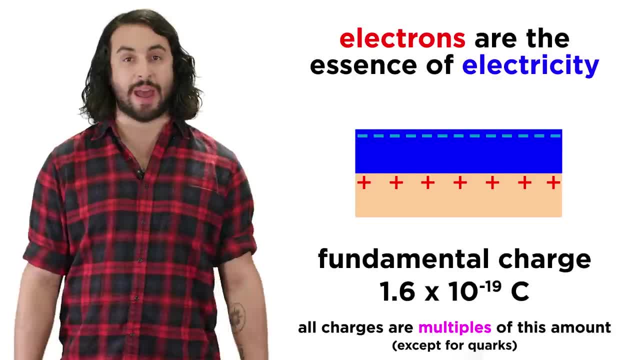 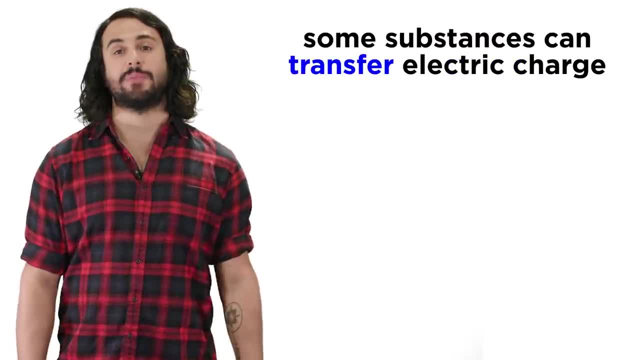 All substances will therefore have a charge that is some multiple of this amount, That is to say, electric charge is quantized. We can categorize substances by their ability to transfer electric charge. A substance that can easily transfer electric charge is a substance that can easily transfer. 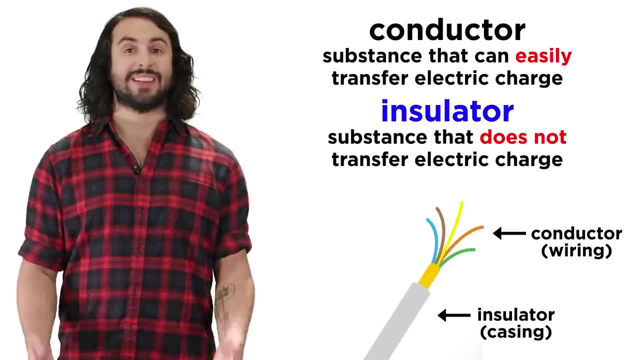 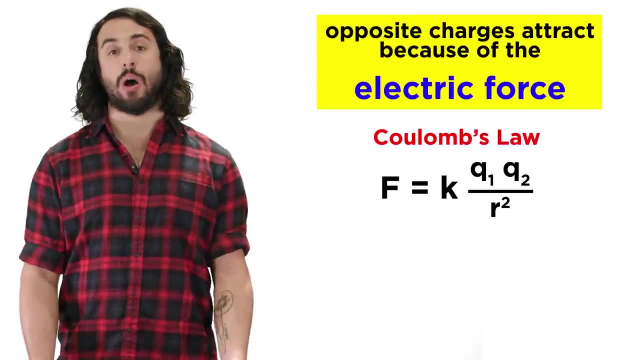 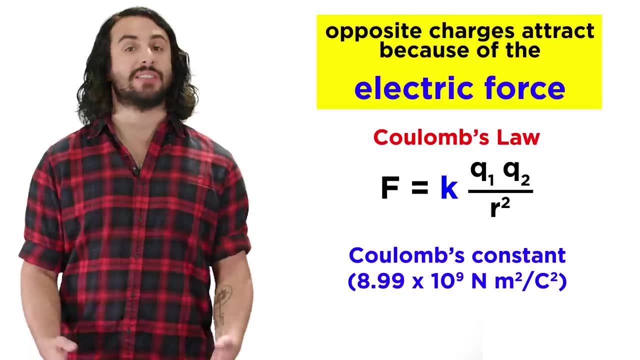 electric charge conductor. one that can't is an insulator. Opposite charges attract one another because of the electric force. This is outlined in Coulomb's law, which states that the magnitude of the electric force between two objects is equal to the Coulomb constant times, the charge on one object times the charge on the other. 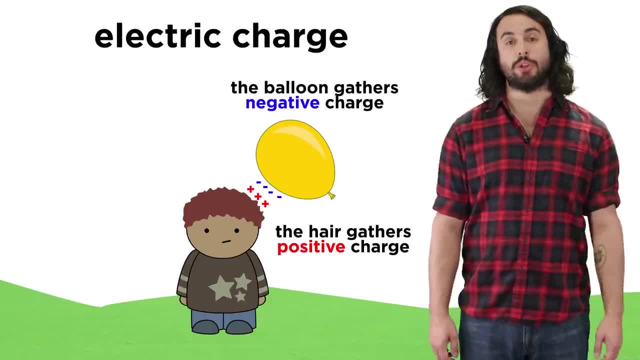 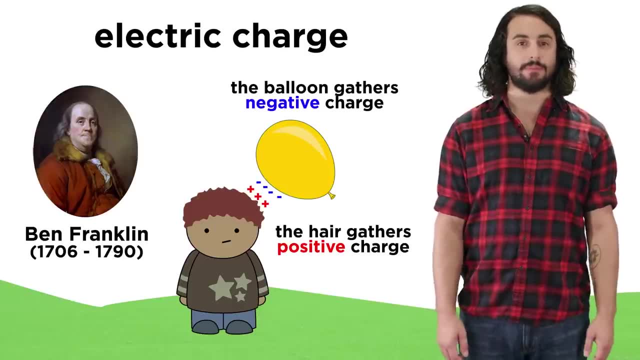 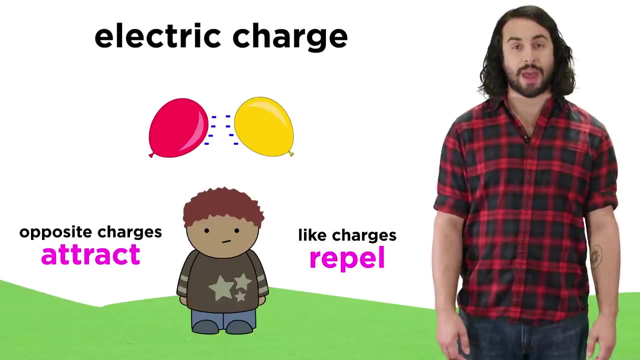 The hair becomes positively charged, and the balloons become negatively charged, which is terminology developed by Benjamin Franklin. Opposite charges will attract one another, which is why your hair sticks to the balloon, and like charges repel, which is why the two balloons push each other away. 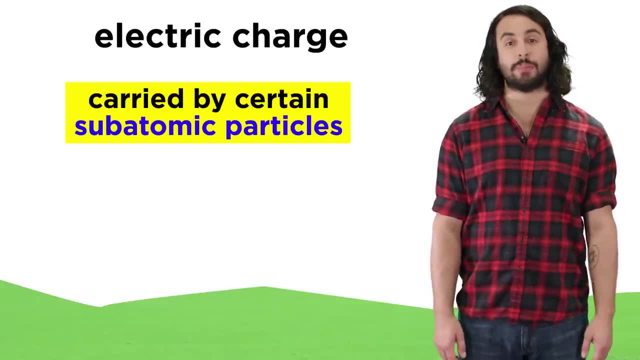 This property of electric charge is carried by certain subatomic particles, the most common of these are protons, which are positive. 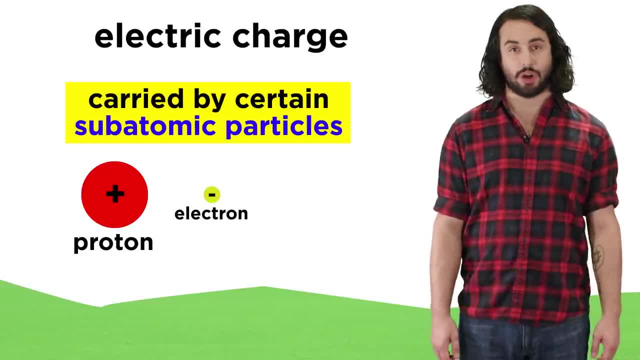 These are positively charged, and electrons, which are negatively charged. Along with neutrons, these make up all the atoms in the universe. 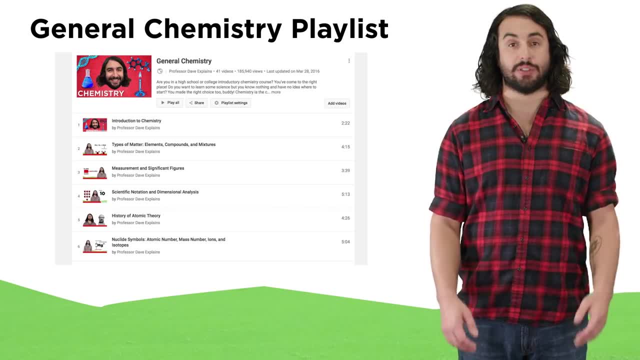 For more about atoms, check out my general chemistry course. 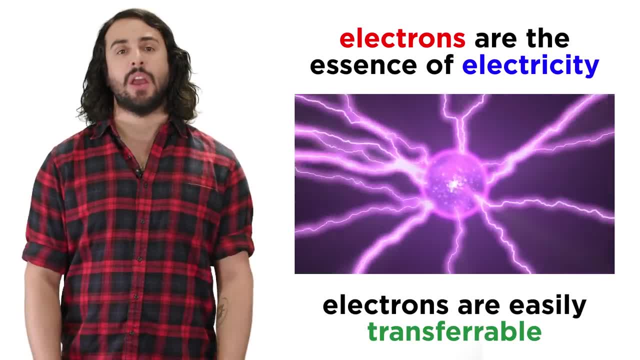 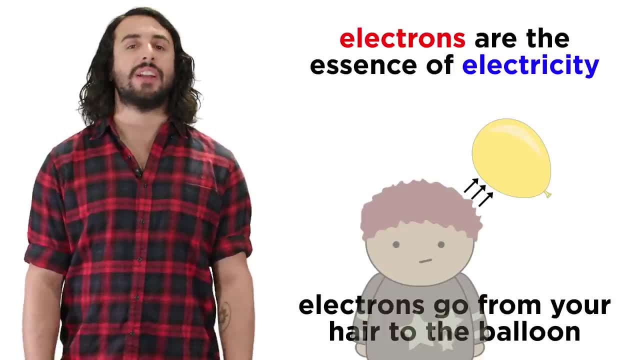 As it happens, electrons, which are the essence of electricity, are easily transferable, and it is the transfer of electrons, in this case from your hair to the balloon, that generates electric charge in previously neutral materials. 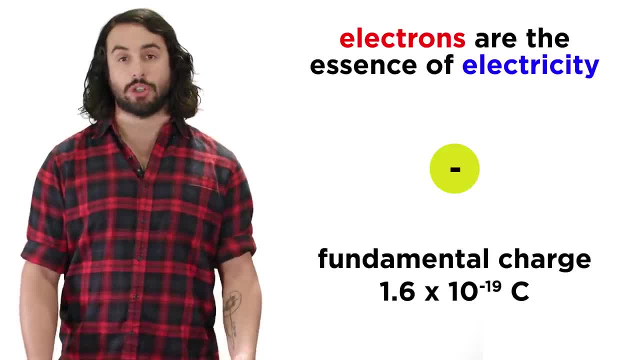 Each electron carries with it the fundamental charge, which is 1.6 times 10 to the negative 19 coulombs. 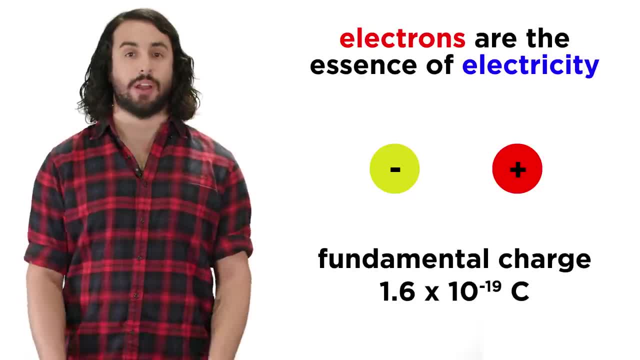 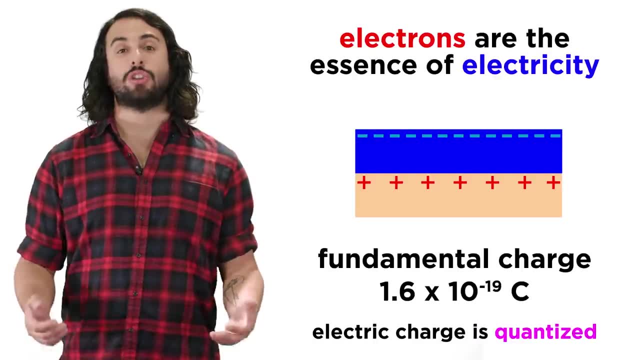 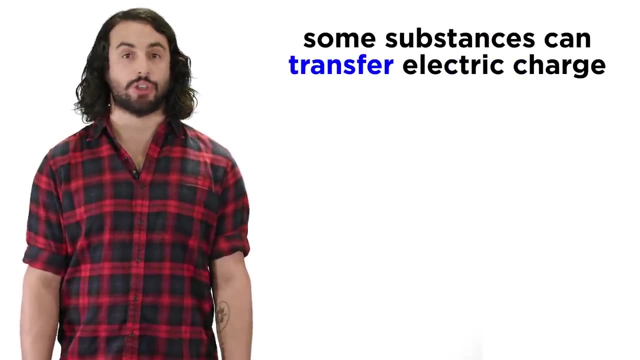 This magnitude is negative for the electron, and positive for the proton. All substances will therefore have a charge that is some multiple of this amount. That is to say, electric charge is quantized. We can categorize substances by their ability to transfer electric charge. A substance that can easily transfer electric charge is a substance that can easily transfer electric charge. 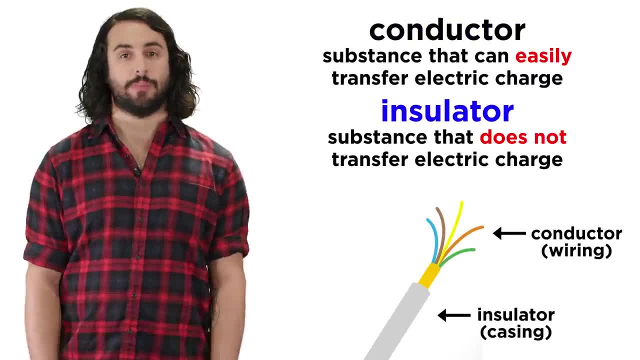 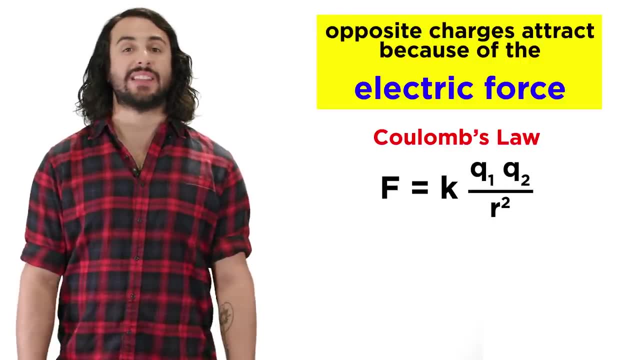 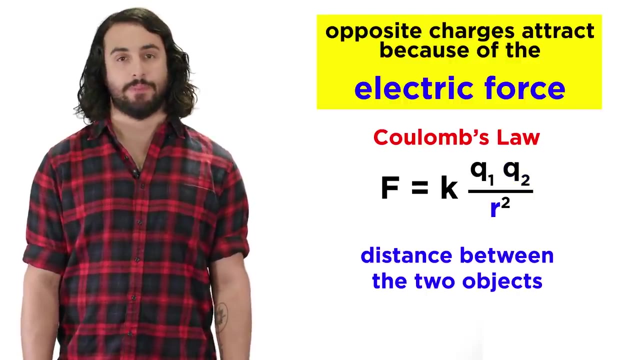 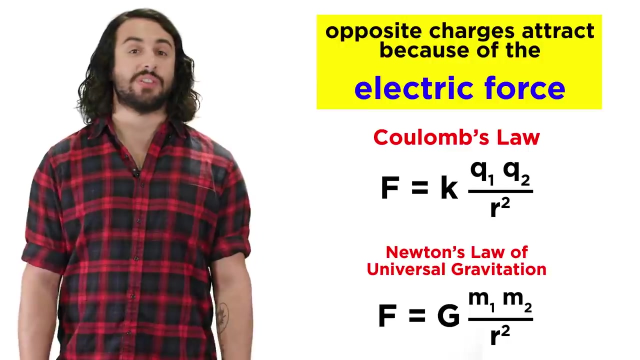 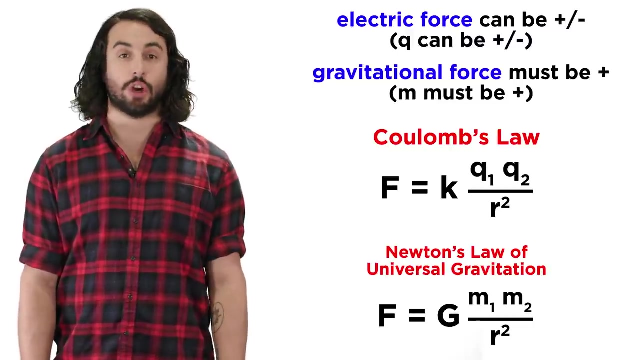 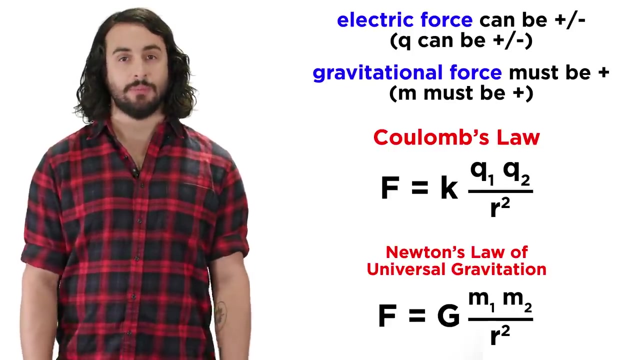 conductor, one that can't is an insulator. Opposite charges attract one another because of the electric force. This is outlined in Coulomb's law which states that the magnitude of the electric force between two objects is equal to the Coulomb constant times the charge on one object times the charge on the other divided by the square of the distance between them. Remarkably this is essentially identical to Newton's law of universal gravitation, the only differences being that the electric force can be attractive or repulsive depending on the signs of these terms and the resulting sign on the force, while gravity is always attractive. Also it is interesting to note that Coulomb's 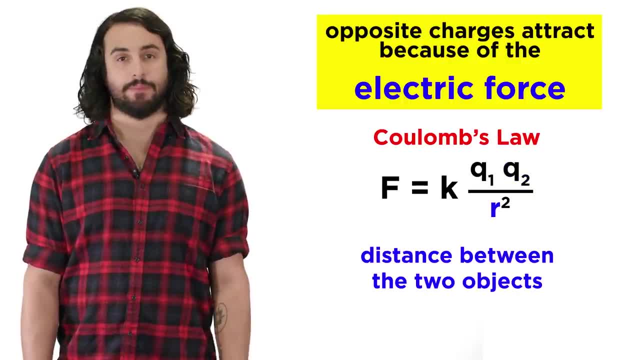 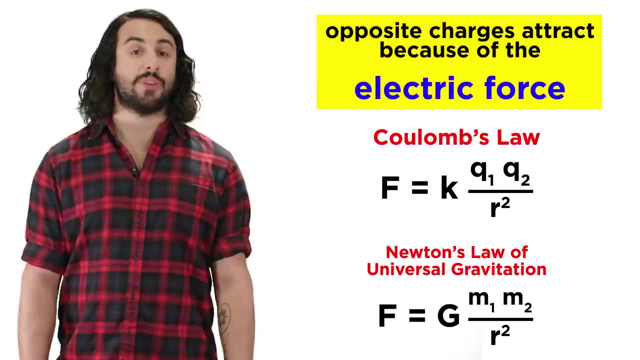 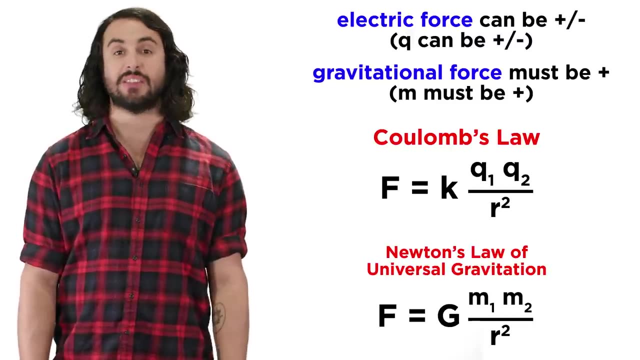 divided by the square of the distance between them. Remarkably, this is essentially identical to Newton's law of universal gravitation, the only differences being that the electric force can be attractive or repulsive, depending on the signs of these terms and the resulting sign on the force. 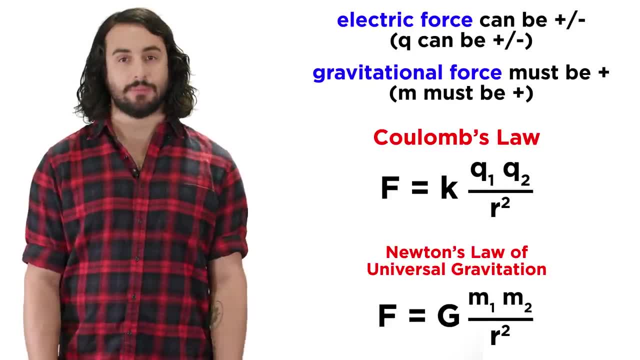 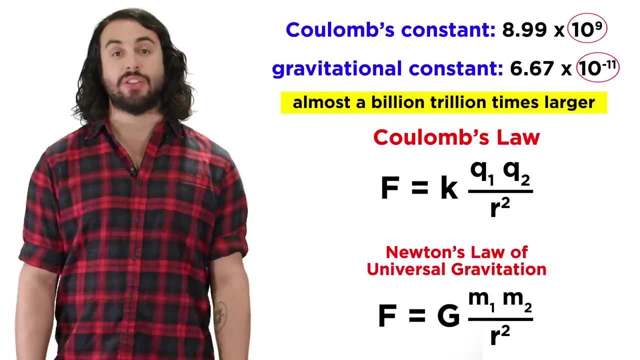 while gravity is always attractive. Also, it is interesting to note that Coulomb's constant is 20 orders of magnitude greater than the gravitational constant, illustrating the discrepancy in gravitation, the strength of the two forces. This law also tells us that the electric force 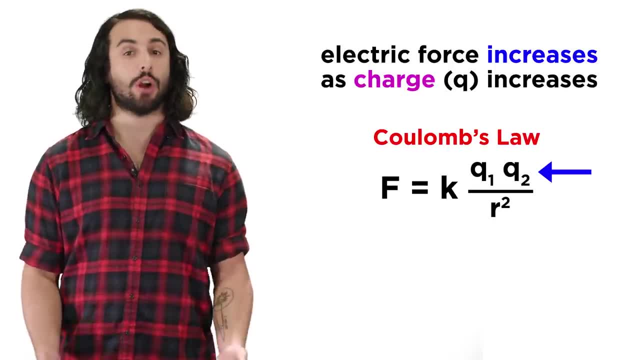 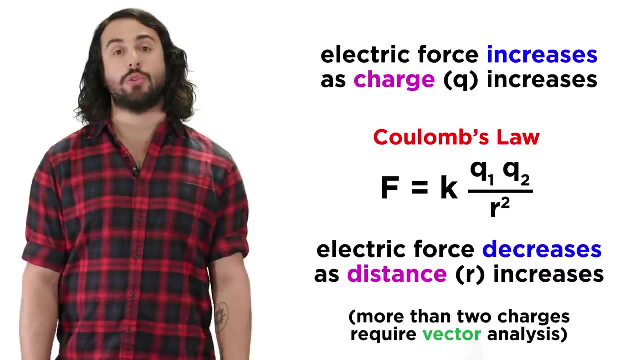 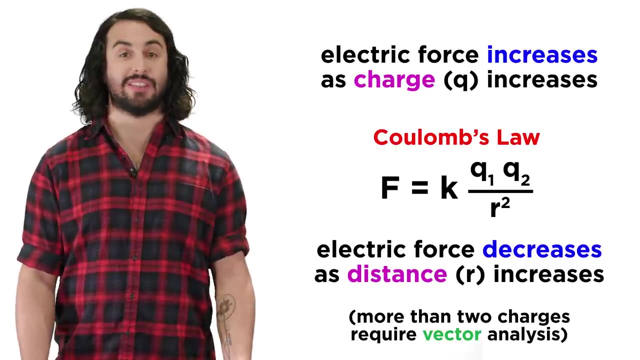 between two objects increases as charge increases and decreases as the distance between them increases. If more than two charges are present, vector addition must be done to find out the net force upon any particle in the system. Just as a gravitational field is what allows the gravitational force to propagate, it is 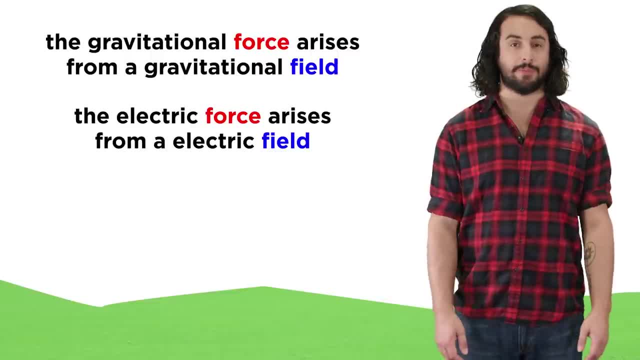 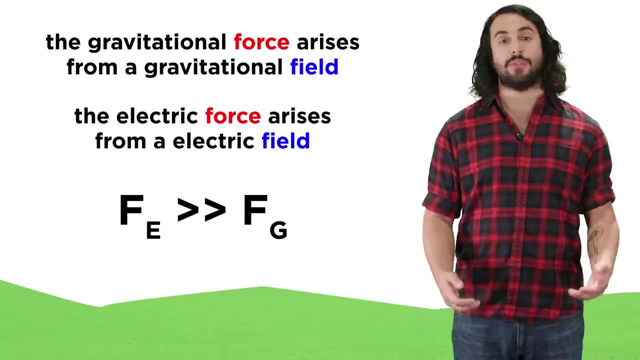 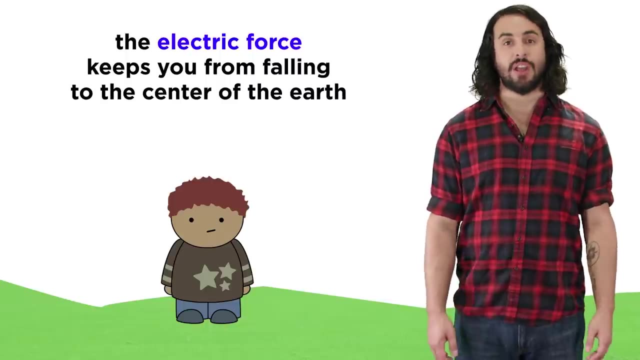 an electric field that allows the electric force to propagate. However, as we said, the electric force is much stronger than gravity. This is evidenced by the fact that the repulsion between particles in your feet and particles in the ground is more than strong enough to keep you from plummeting towards the center of the. 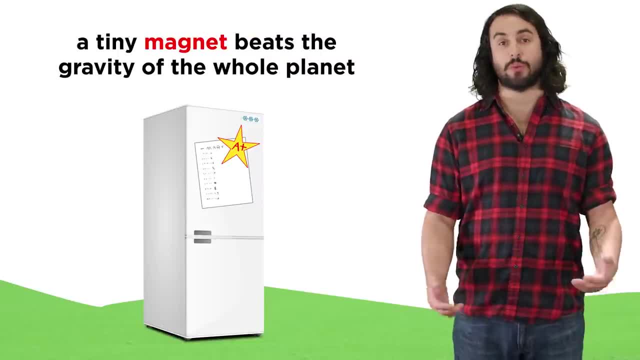 earth. We can also use a cheap refrigerator magnet to keep a piece of paper on the fridge against the gravitational pull of the entire planet. We can also use a cheap refrigerator magnet to keep a piece of paper on the fridge against the gravitational pull of the entire planet. 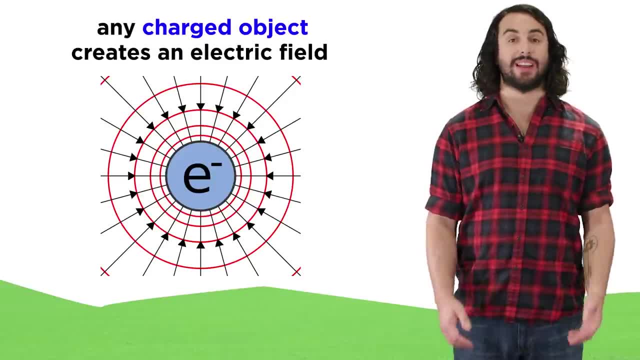 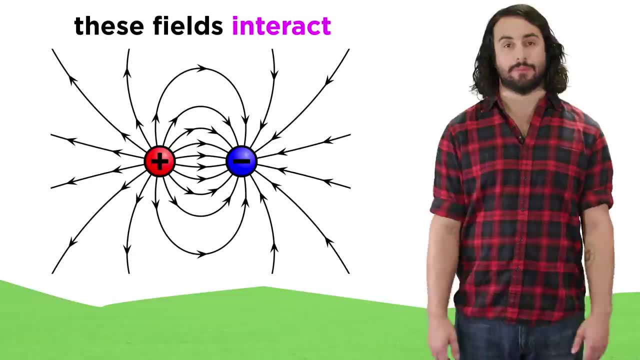 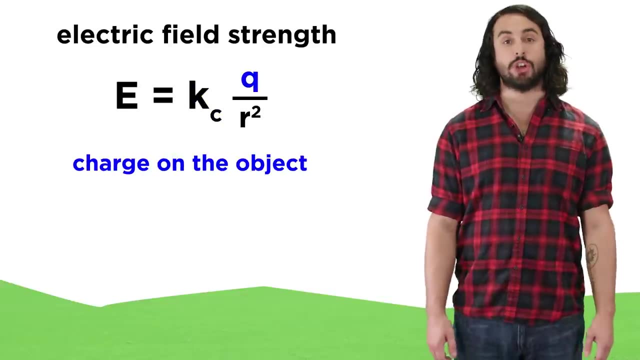 planet. Any charged object will manifest an electric field around itself and if another charged object enters this field, interactions will occur. The strength of an electric field generated by a point charge is equal to the Coulomb constant times the charge on the object producing the field divided by the square of the distance. 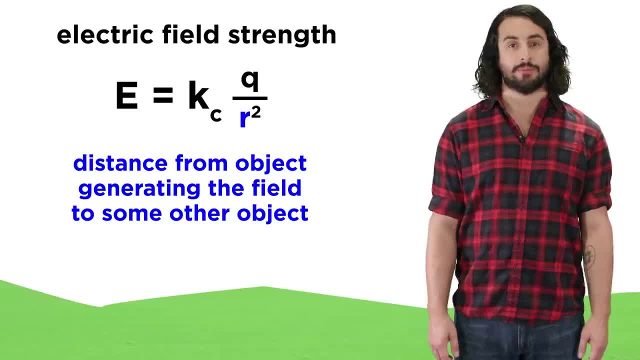 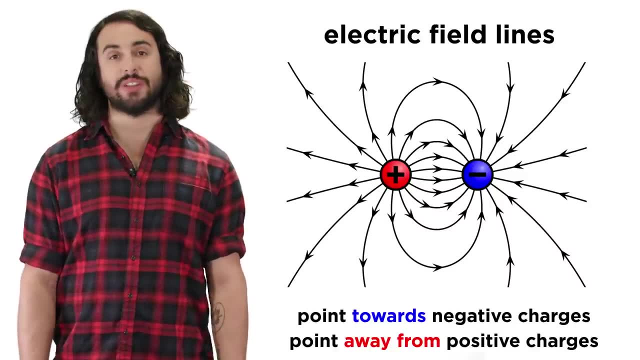 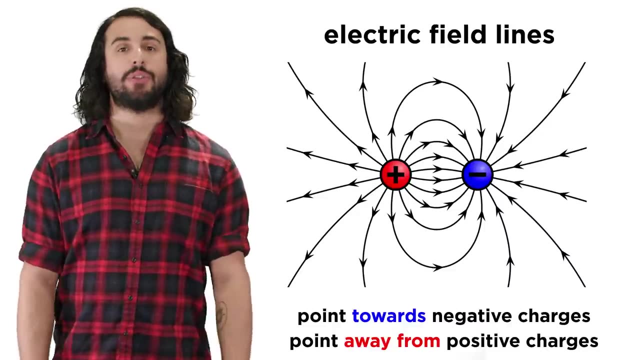 between this object and whatever it is acting on. One way we depict electric fields is by drawing electric field lines, which generally point towards negative charges and away from positive charges and do not cross. These don't really exist, but they are a convenient way to analyze the direction of 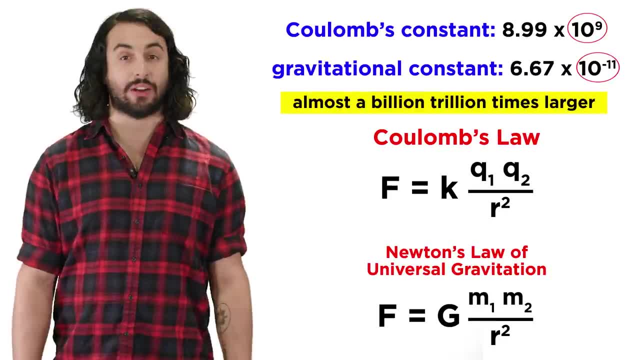 constant is 20 orders of magnitude greater than the gravitational constant, illustrating the discrepancy in gravitation. 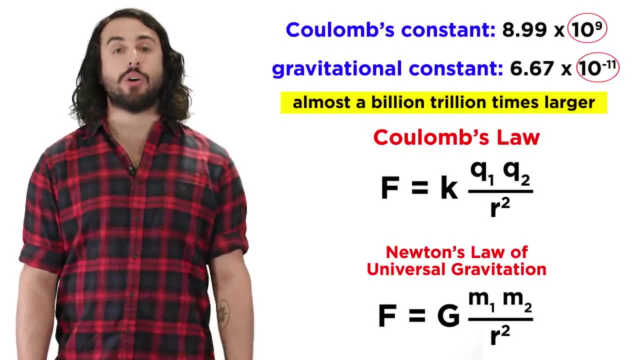 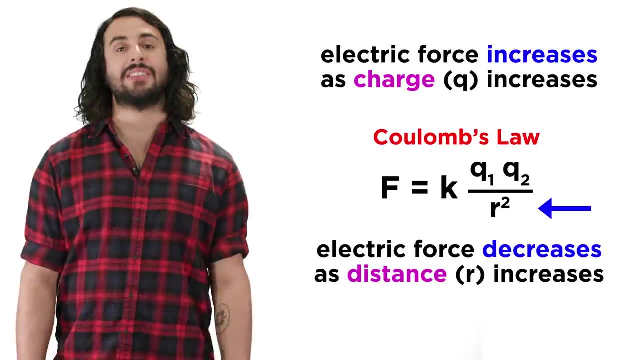 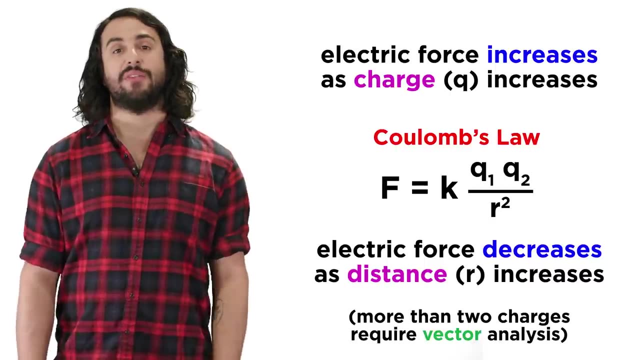 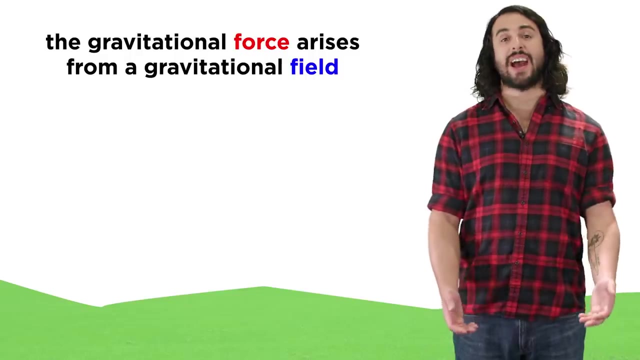 the strength of the two forces. This law also tells us that the electric force between two objects increases as charge increases and decreases as the distance between them increases. If more than two charges are present, vector addition must be done to find out the net force upon any particle in the system. Just as a gravitational field is what allows the gravitational force to propagate, it is an 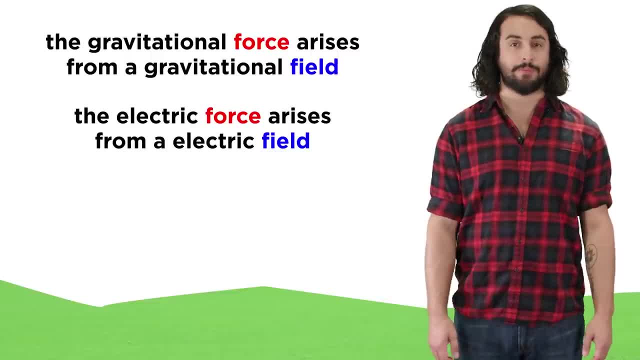 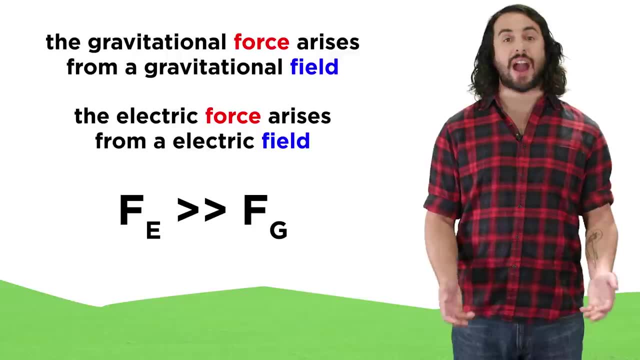 electric field that allows the electric force to propagate. However, as we said, the electric force is much stronger than gravity. This is evidenced by the fact 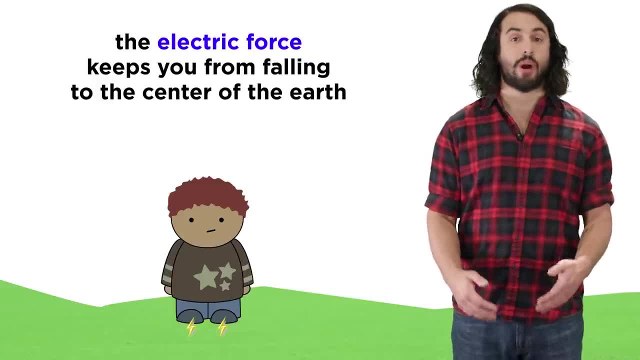 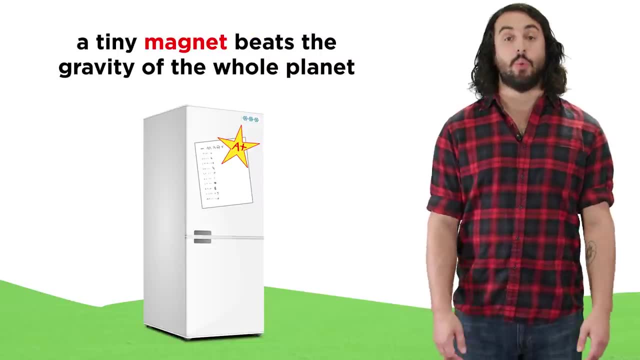 that the repulsion between particles in your feet and particles in the ground is more than strong enough to keep you from plummeting towards the center of the earth. We can also use a cheap refrigerator magnet to keep a piece of paper on the fridge against the gravitational pull of the entire plane. 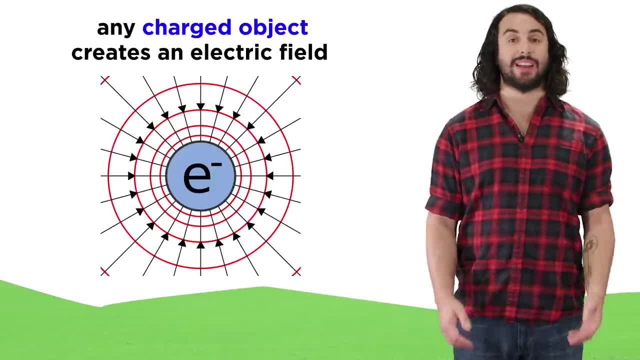 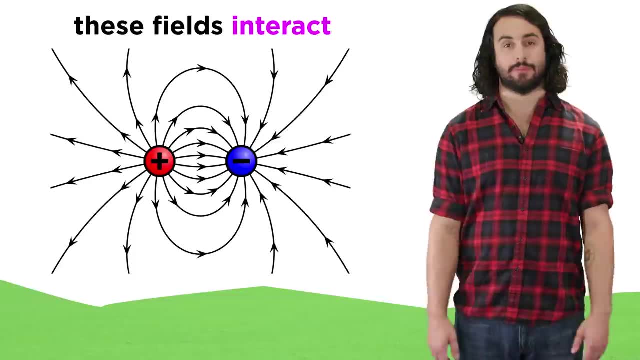 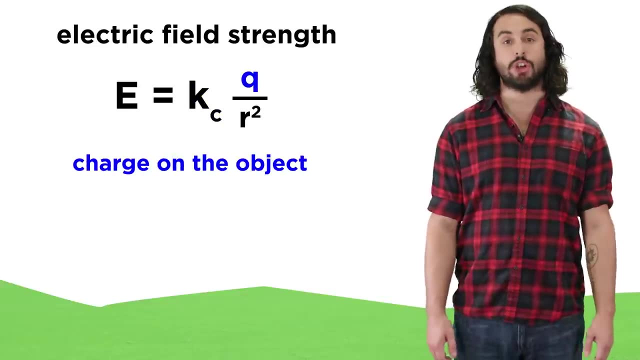 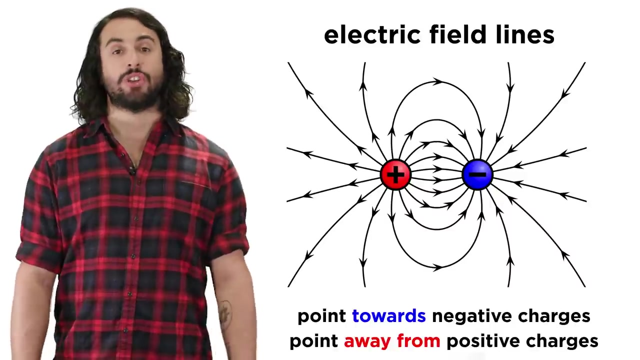 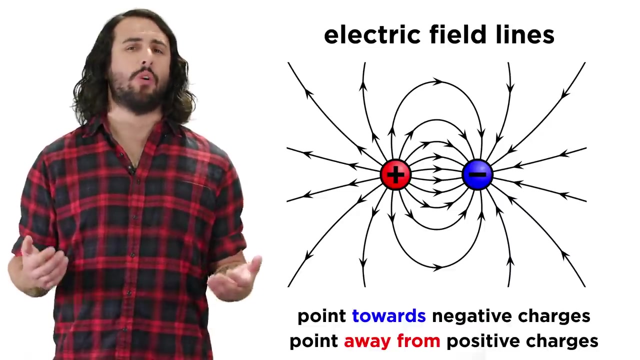 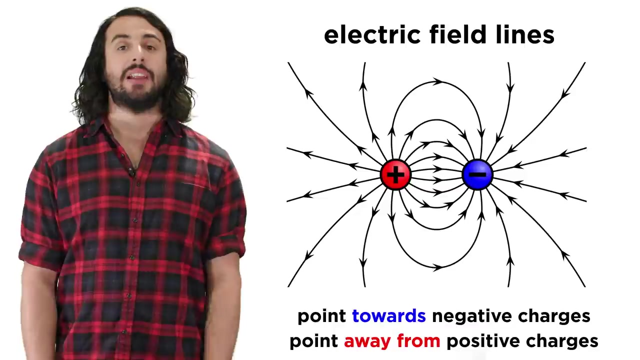 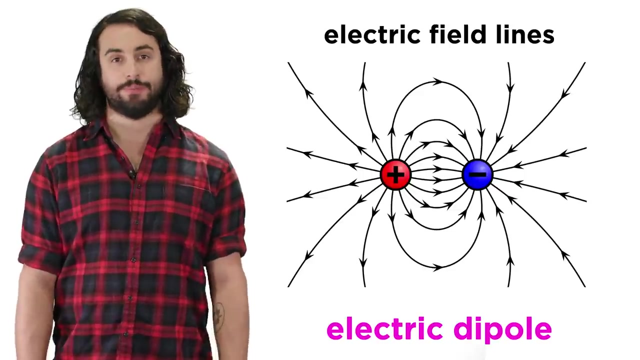 planet. Any charged object will manifest an electric field around itself, and if another charged object enters this field, interactions will occur. The strength of an electric field generated by a point charge is equal to the Coulomb constant times the charge on the object producing the field, divided by the square of the distance between this object and whatever it is acting on. One way we depict electric fields is by drawing electric field lines, which generally point towards negative charges and away from positive charges, and do not cross. These don't really exist, but they are a convenient way to analyze the direction of a field at any point in space, like the field produced by these two oppositely charged particles, which we can call an electric dipole. 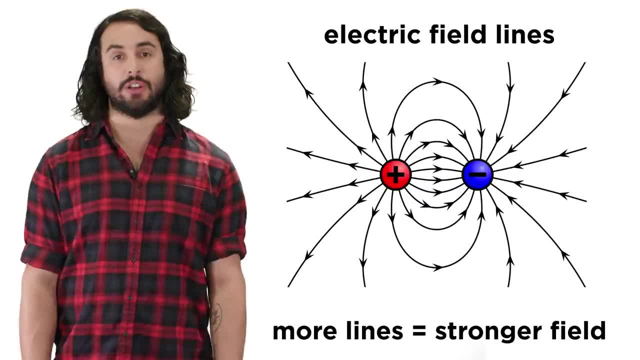 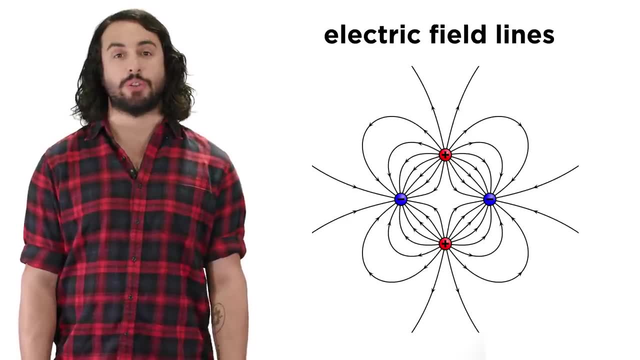 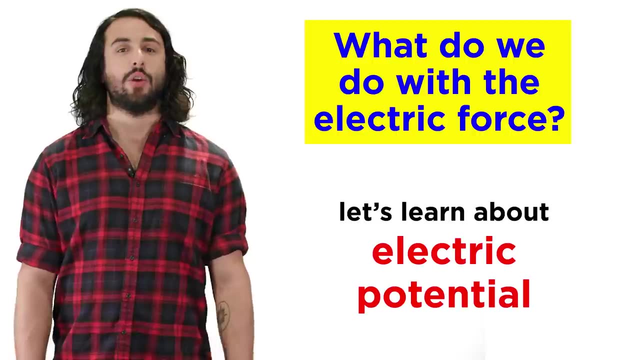 The more densely packed the field lines are in a particular region, the more likely they are, the greater the strength of the field. Lines like these can be especially useful if many particles are producing the field. How is it specifically that we use the electric force to our advantage? To find out, we have to move on to electric potential, but first, let's check comprehension.